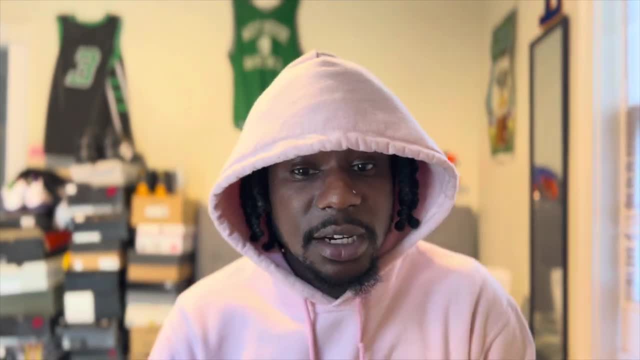 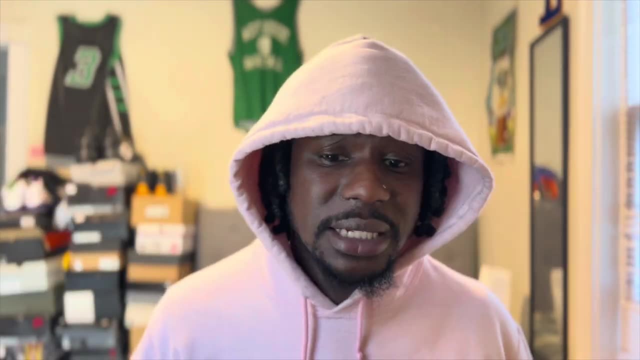 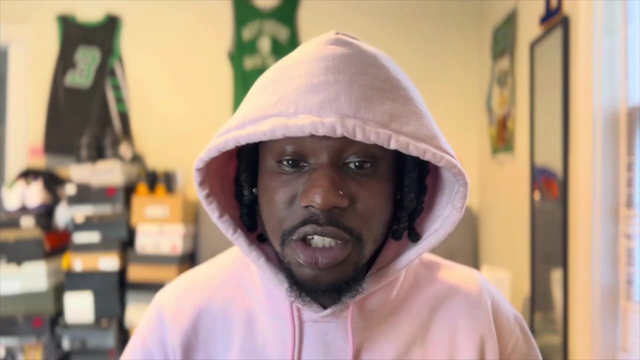 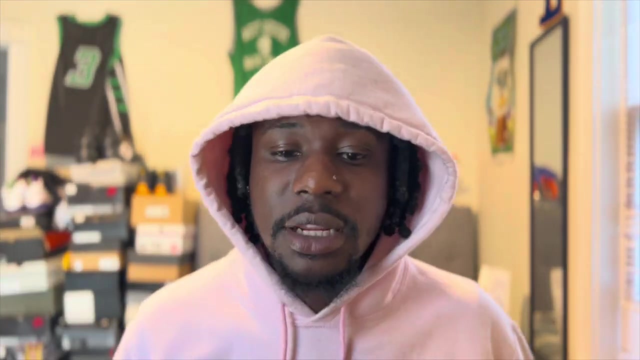 Boogie B, okay, so he's currently incarcerated. he currently like you feel me. so I guess this is a big thing, cause everybody's like, oh shit, I heard he got life, you feel me. so everybody's like, oh shit, he has life, he got life. how the hell he drop? um, I'm assuming he had an actor in this shit, obviously. so we about to see what's up. um, I'm really not sure. yo, OFB got 237, 1516 million, 18,016 million freaking rappers. my nigga, bro, you feel me. so this is a new nigga to me, bro, you feel me? so? 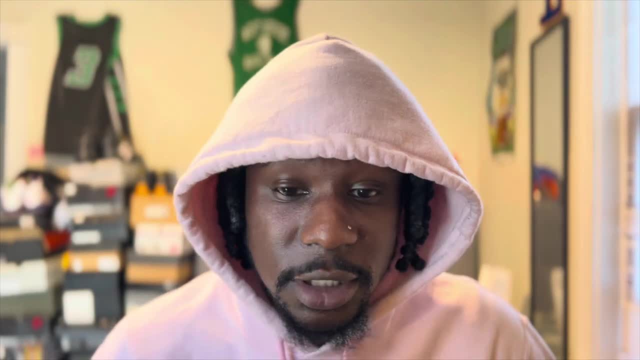 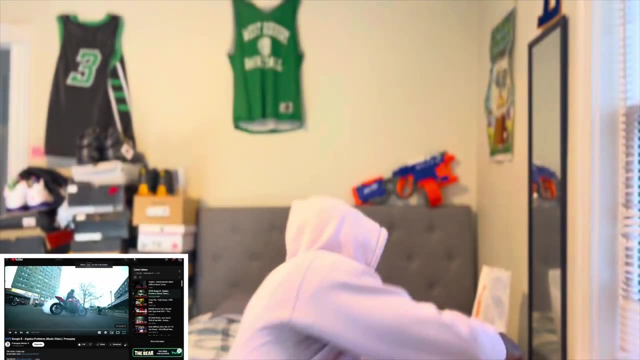 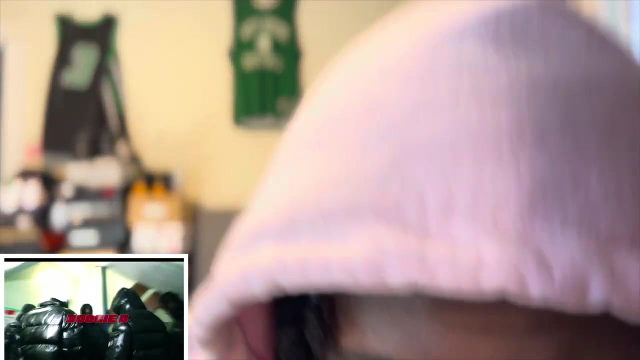 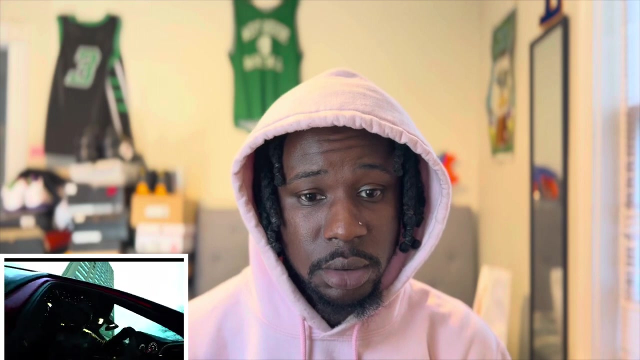 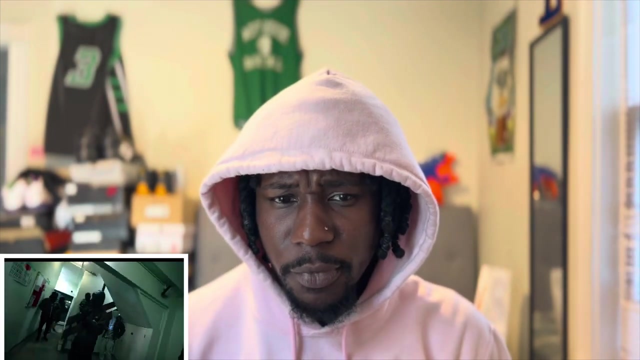 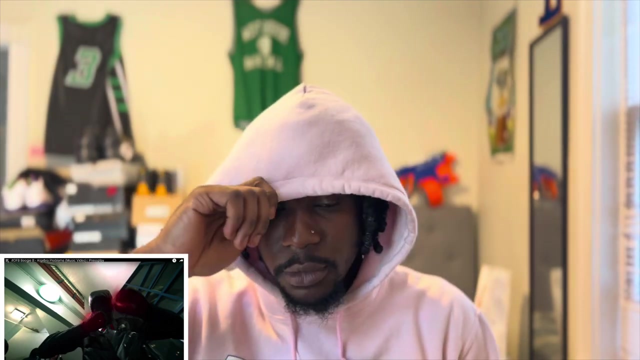 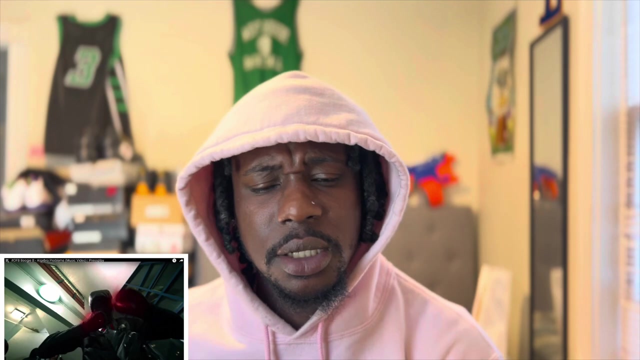 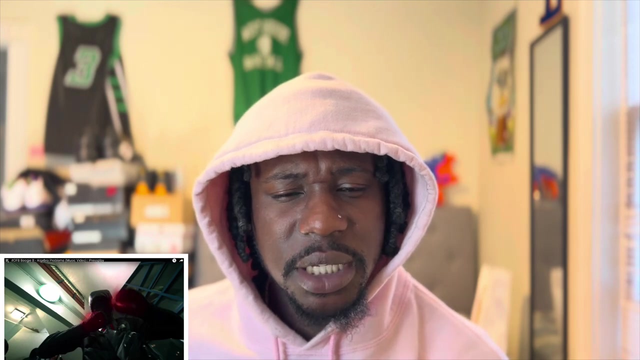 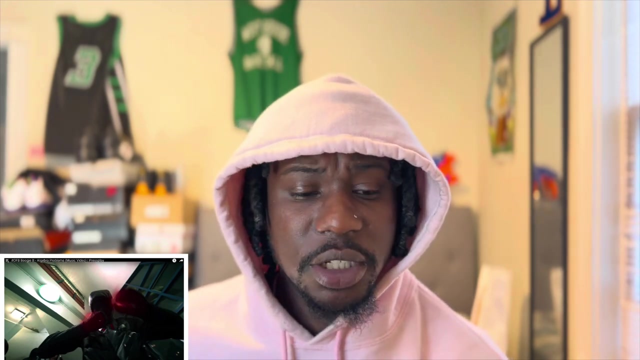 let's get to it. man two days ago, um shit, 40k views. let's get to it, guys, let's go. let's get to it. man two days ago, um shit, 40k views. let's get to it, guys, let's go. 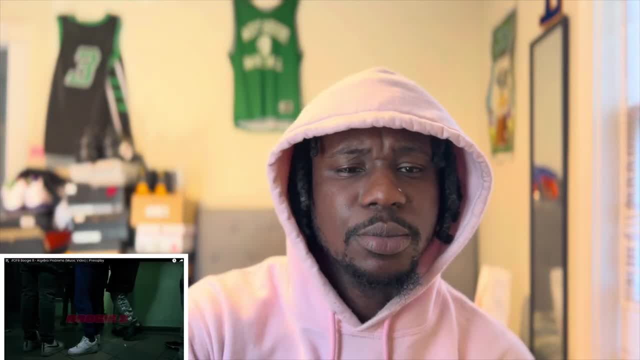 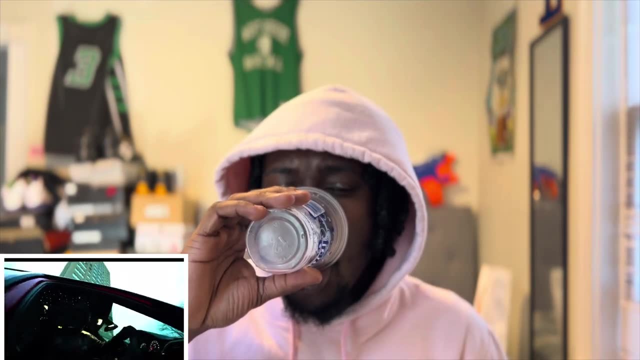 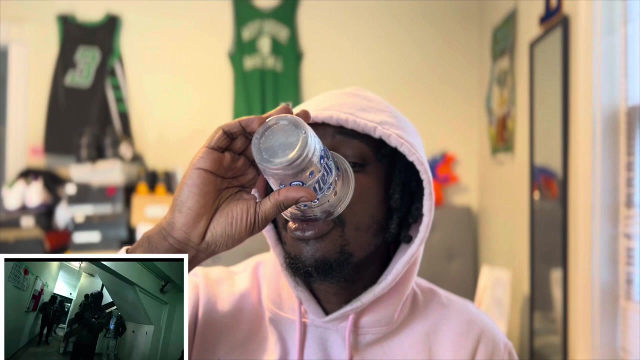 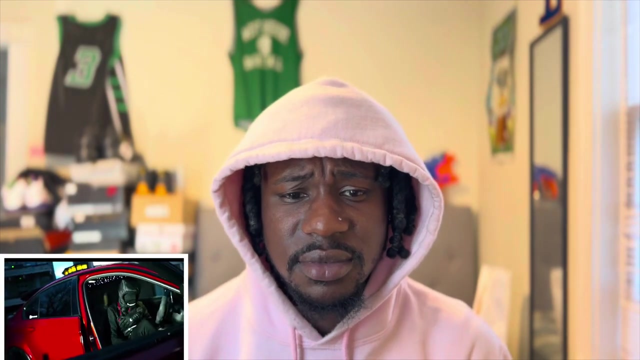 let's get to it. man two days ago, um shit, 40k views. let's get to it, guys, let's go. let's get to it. man two days ago, um shit, 40k views. let's get to it, guys, let's. 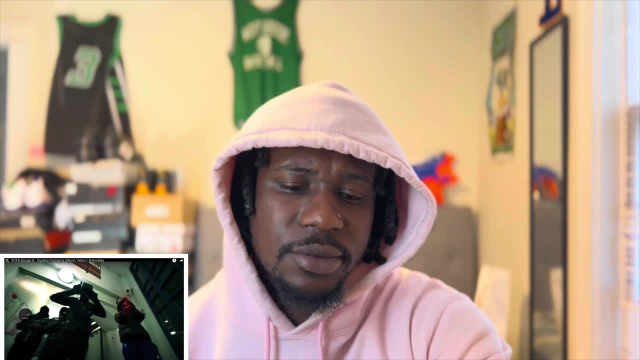 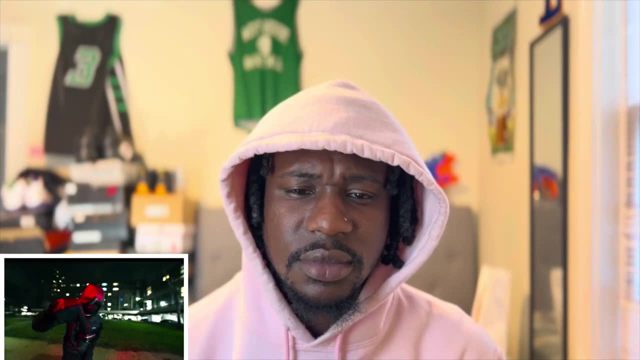 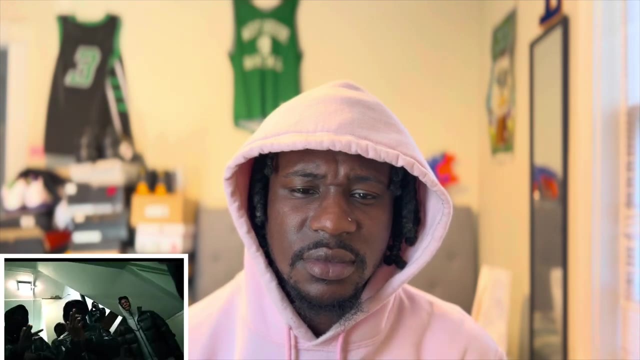 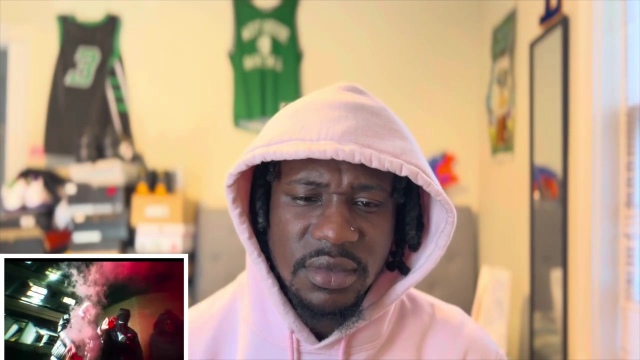 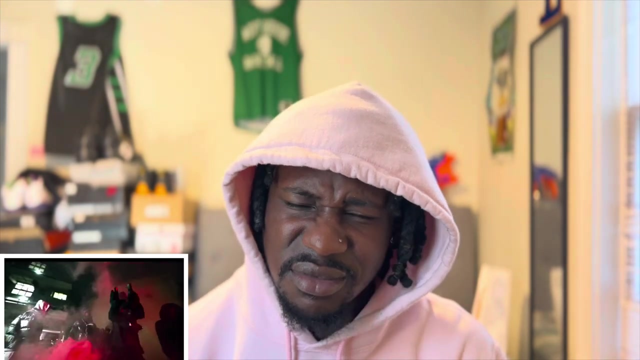 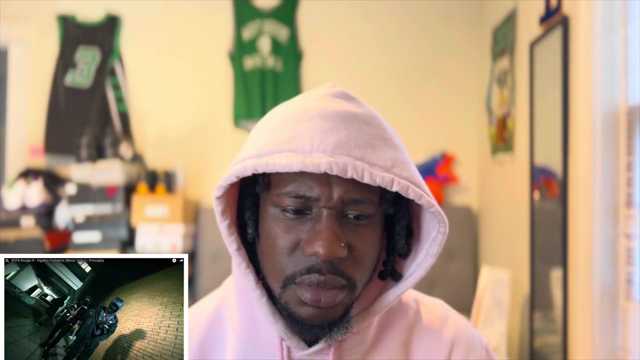 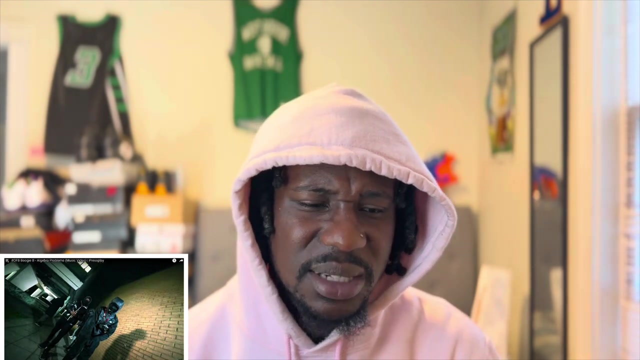 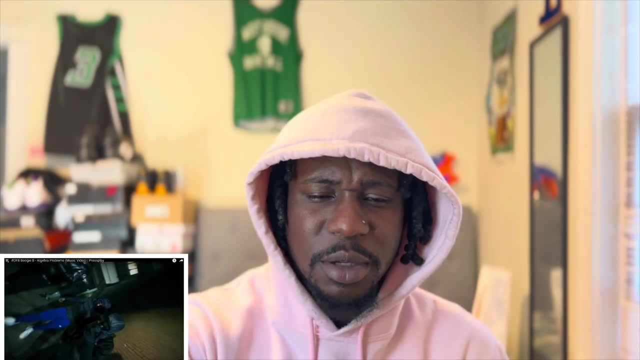 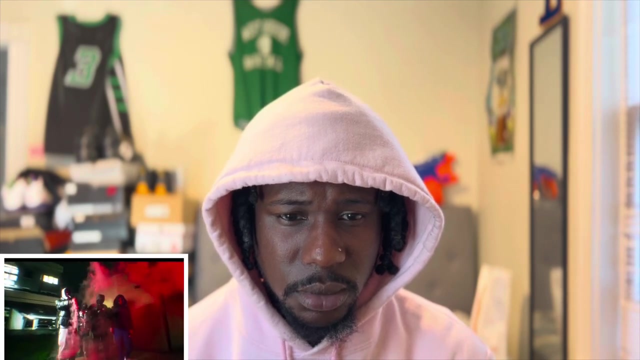 get to it, man two days ago, um shit, 40k views. let's get to it, guys, let's get to it. let's get to it. man two days ago, um shit, 40k views. let's get to it, guys, let's get to it. 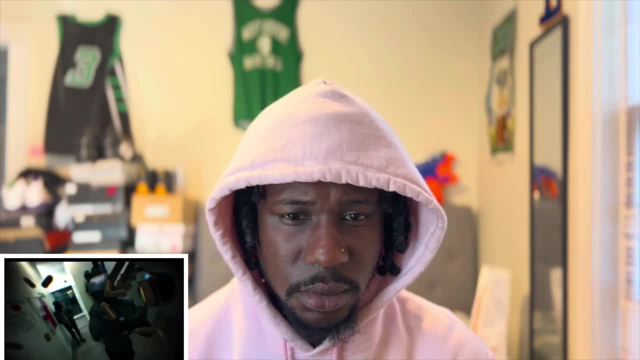 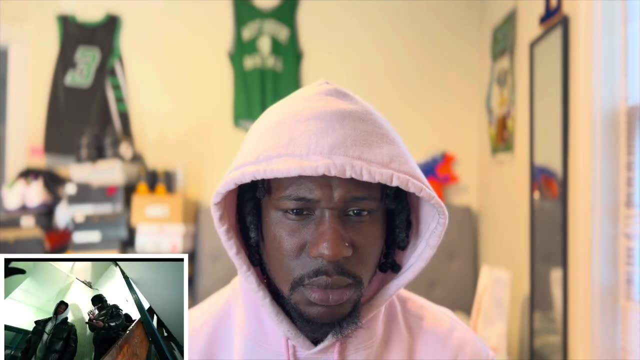 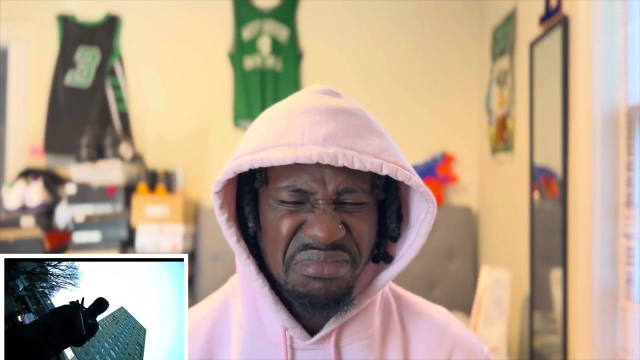 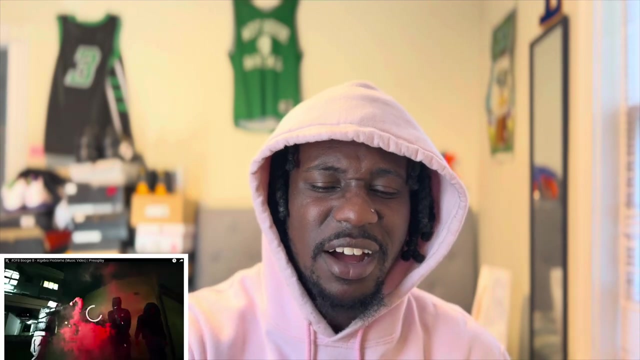 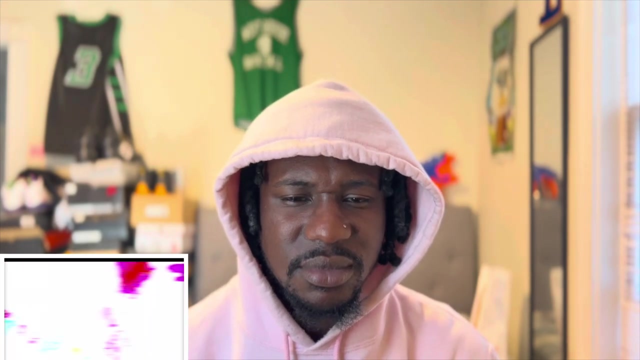 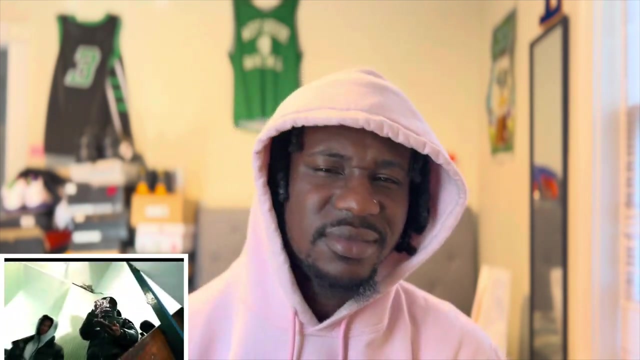 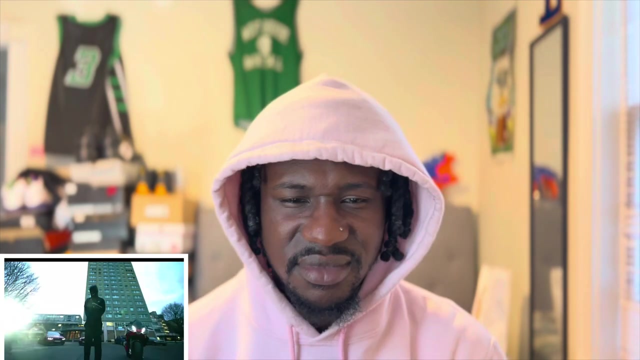 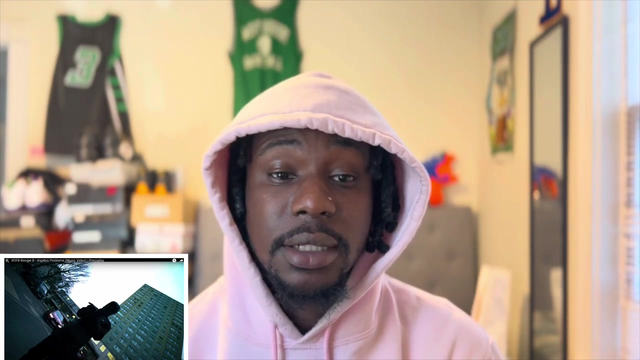 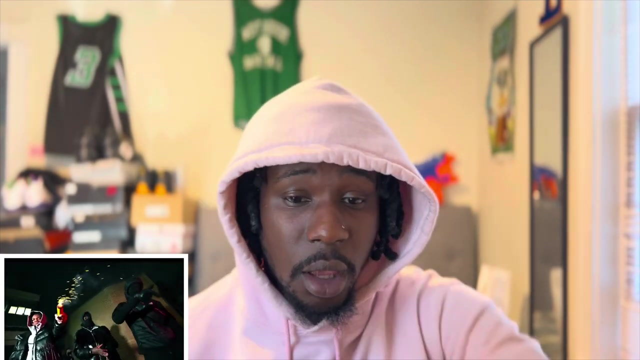 let's get to it. man. two days ago, um shit 40k views. let's get to it, guys, let's get to it. let's get to it. man, two days ago, um shit 40k views. let's get to it, guys, let's get to it. 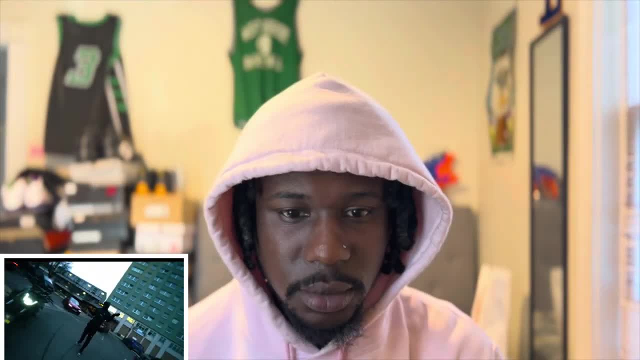 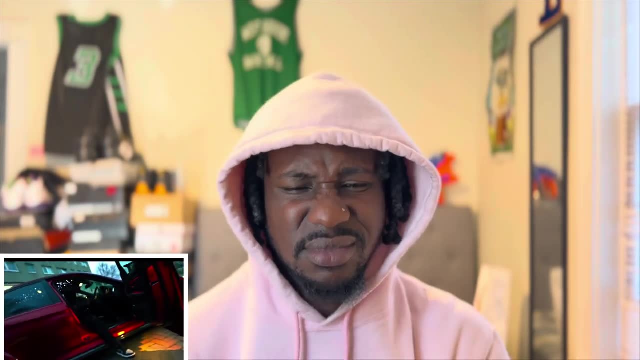 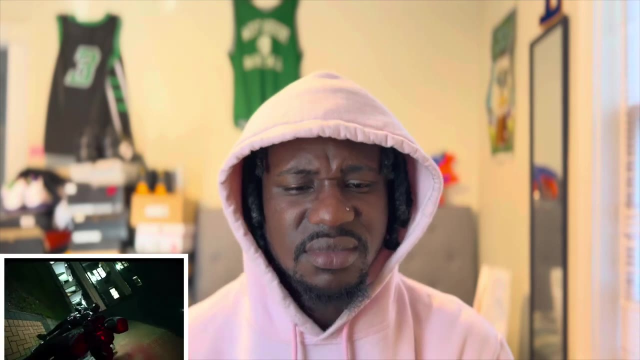 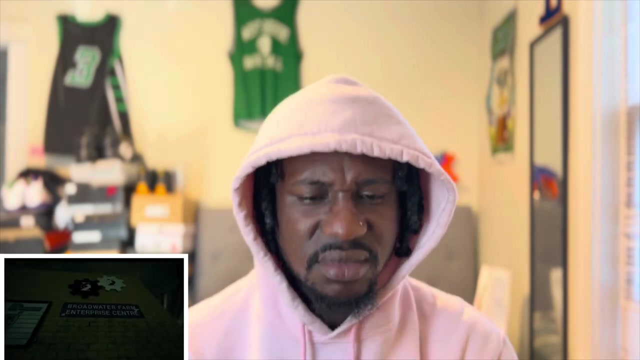 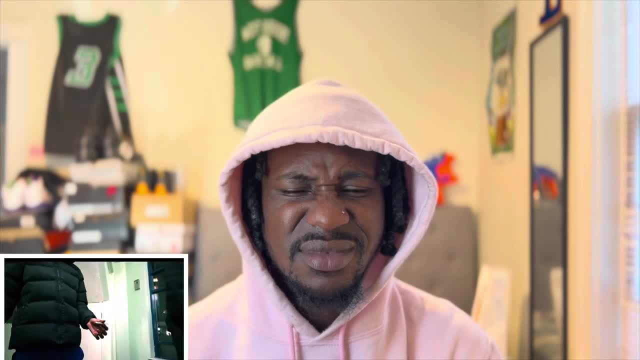 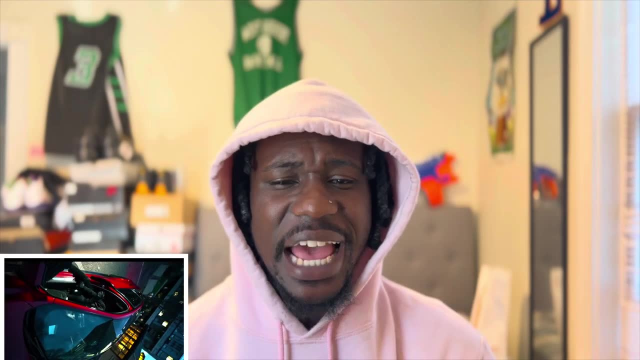 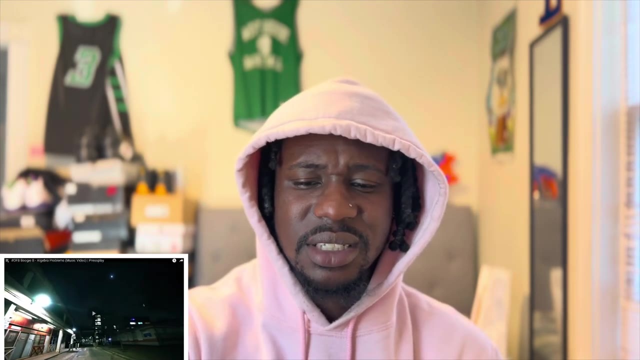 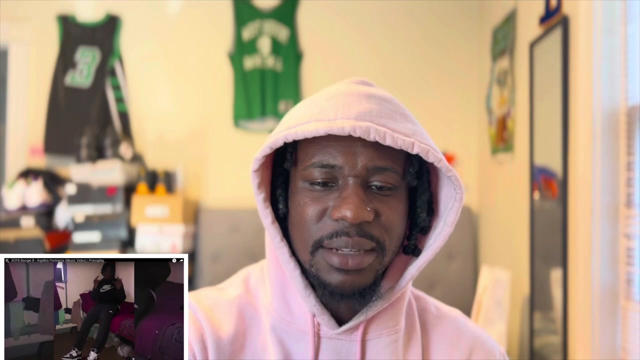 I don't know. I don't know if I'm jacking this for real, because I don't know. I don't think I'm jacking this. Is it more? Yeah, free, Damn, he got them LV sneakers in the unit too.